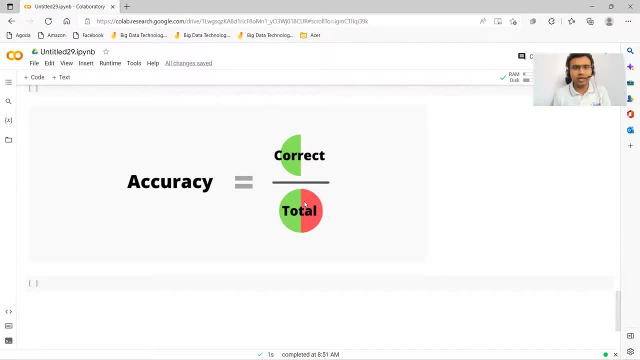 the accuracy in percentages. if i find so, i'll just multiply it by 100, then i will get it into percentages. so what i can simply do is i can here start with from. so sklearn we have, sklearn has got packages for everything. okay, so from sklearn dot metrics. so i need which packages? metrics packages. 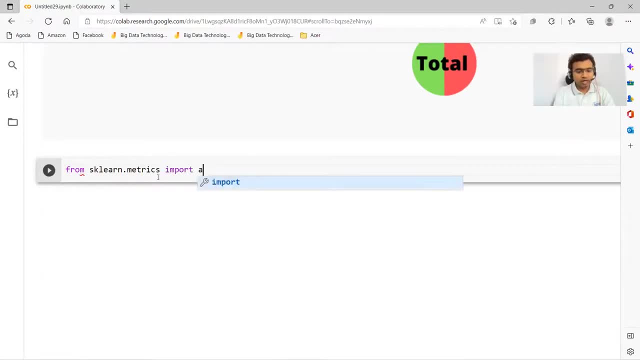 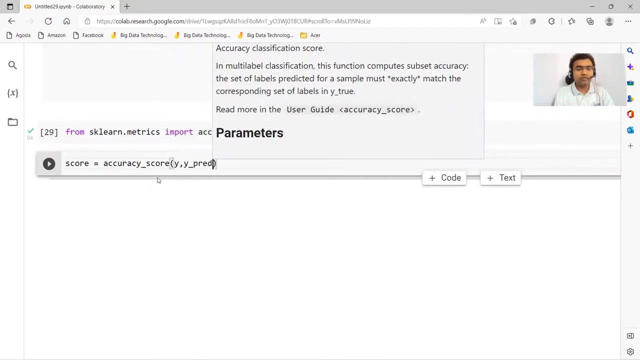 so from sklearn dot metrics import accuracy score. so accuracy score will help me to compute this now. s-c-o-r-e score is equal to accuracy score and i will pass here two things. and first thing is the y, which we all know already have, and y underscore pred, which the algorithm has made. and now let me display. 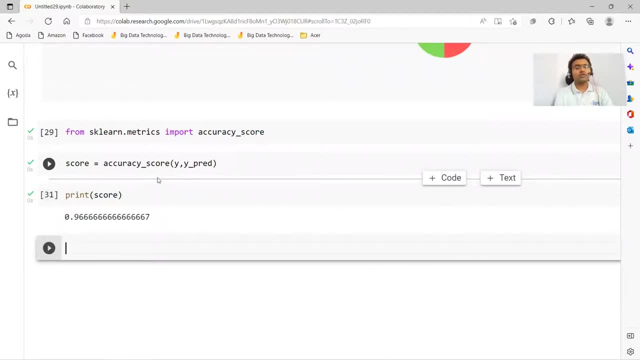 that, what score do we have for accuracy? so 0.9666, that means 96.7 percent, is the accuracy. that is the accuracy the model has given. so this is how we can find the accuracy. now this sklearnmetrics has got multiple packages, so I will just show you and which we will be discussing. 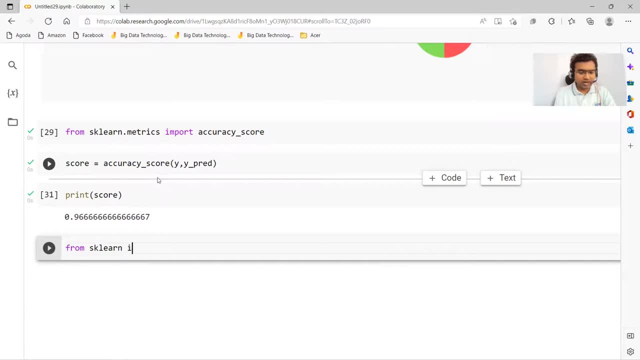 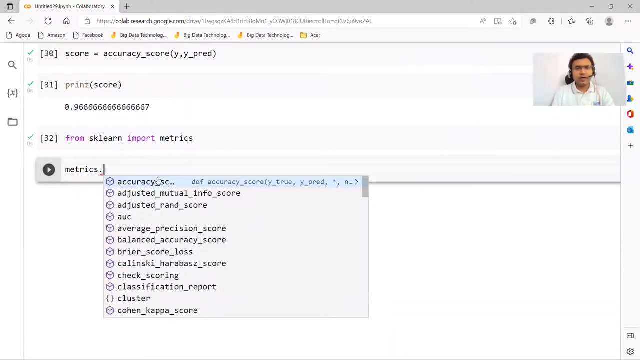 on further discussions. so from sklearn I can do import, import matris, matrix. so this matrix has got multiple packages. now if I do metrics dot, so it is going to show me the list of formulas, the functions it is having, so you can see accuracy score. then we have 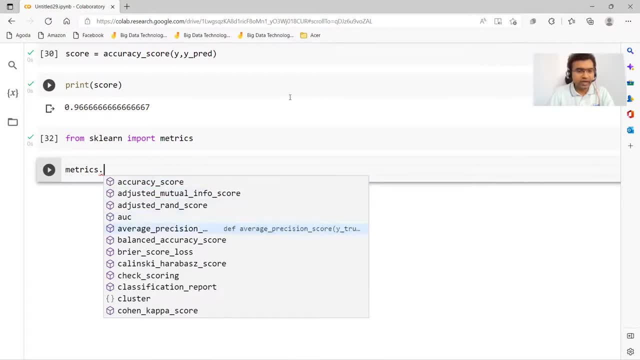 pronounced values like x, y and x, y and tan, x, y, and so it has got multiple packages. so adjusted mutual info, adjusted RAND score, AUC, average precision score, balanced accuracy, Breer score, So multiple scores. it has got confusion. matrix it has. 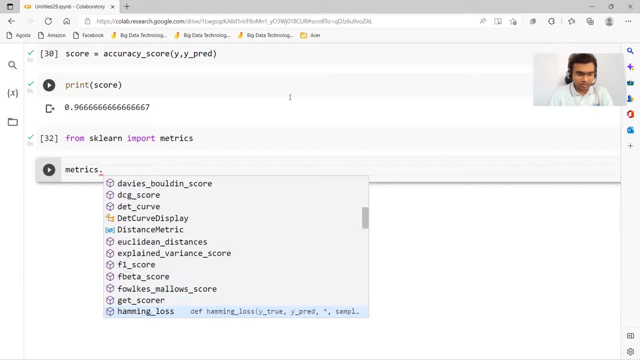 got. So these things we can use with different different algorithms. Okay, so they have relevance with respect to different different algorithms, the type of algorithms we have. So matrix is very powerful for identifying the accuracy of a model, So you can use this. 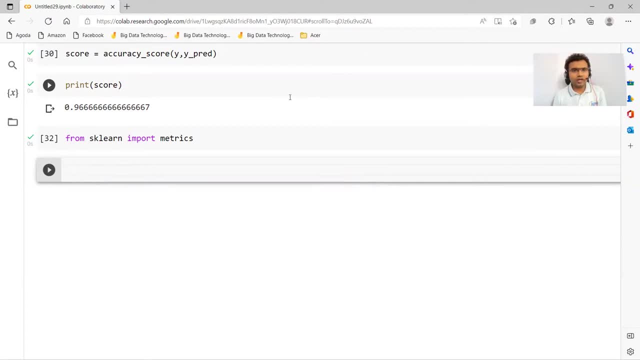 So that's it for this particular video. Now you can build your algorithms And after that, build means what? So you are not exactly building your algorithms, You are just creating, using the packages and making the algorithms implemented or getting them trained, and then